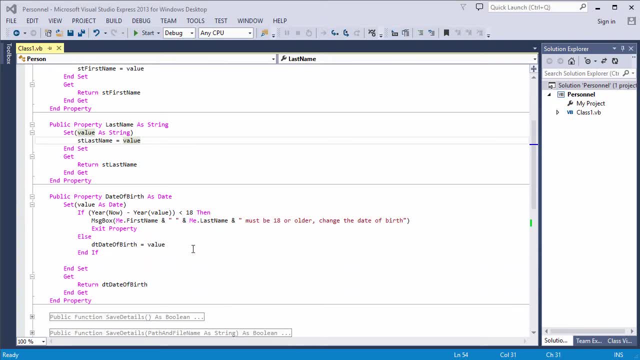 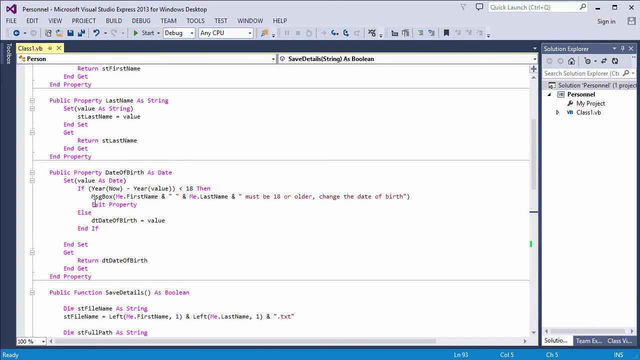 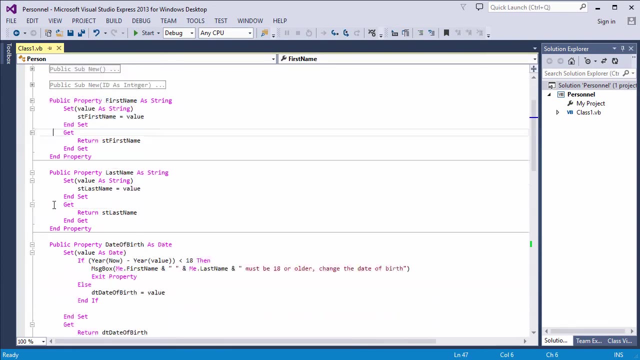 with first name, last name and date of birth properties. There's also a saveDetails method. In fact, I've got several overloads of it And I've got a customized constructor and I've overloaded this as well. Let's remind ourselves of the front end. 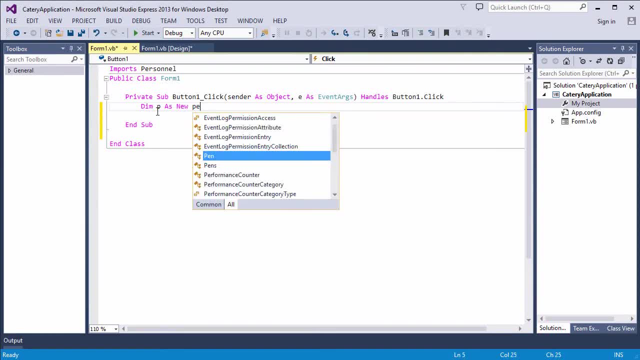 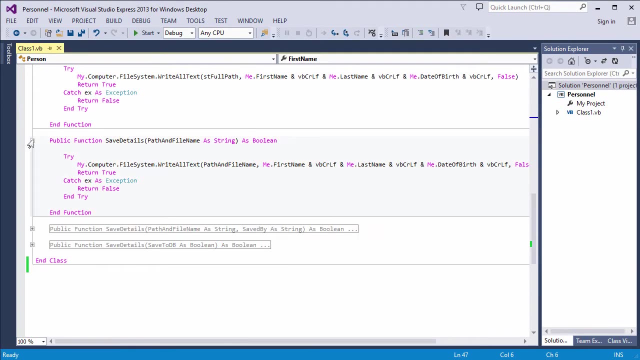 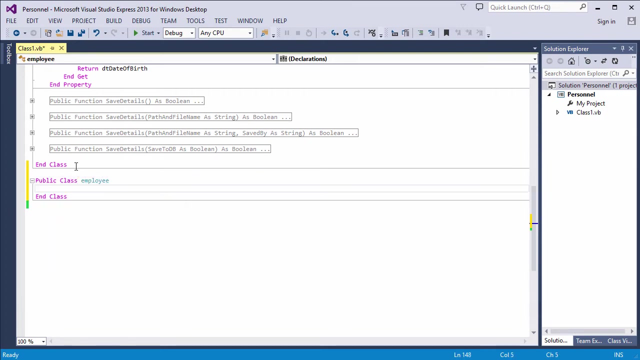 I can create a new person object and I can set various properties and call the methods. That'll do for now. Let's write an employee class. I'm writing the code inside the same class library project as the person class, So my employee class will also be compiled into personneldll. 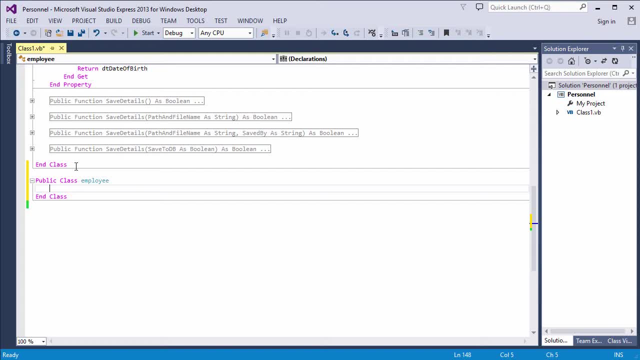 An employee is a type of person with a first name, a last name, a date of birth, etc. So I'm going to inherit all of the properties and methods from person, just like this. Now I'm going to build the library. 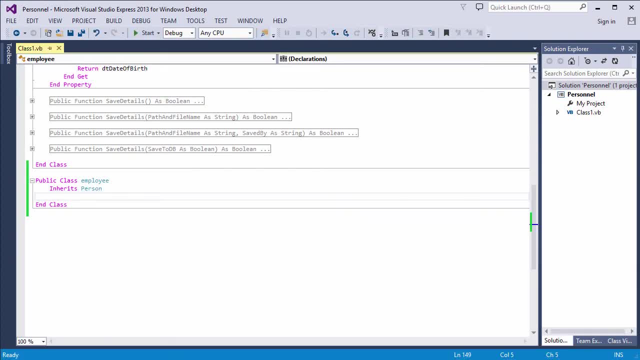 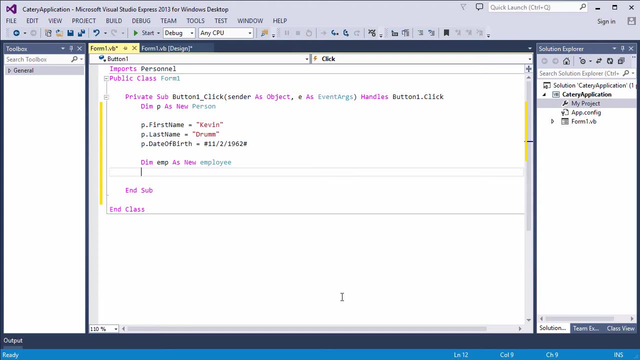 And let's see what we can do at the front end. now. Notice: I used emp instead of e because the button procedure is already being passed a parameter called e as event arguments. My employee now has all of the properties and methods of a person. 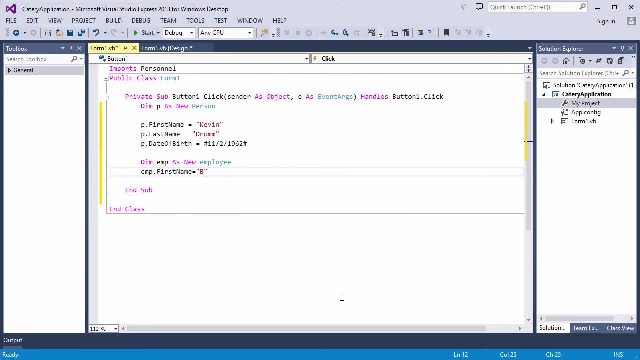 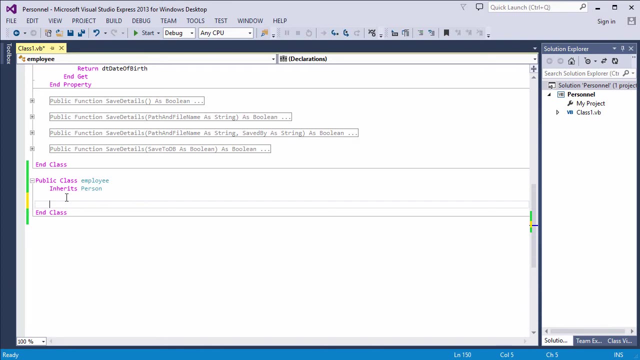 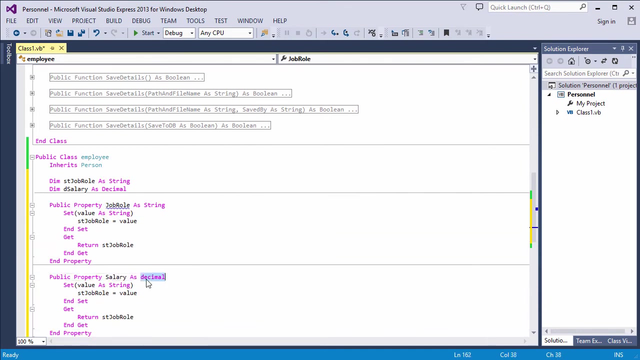 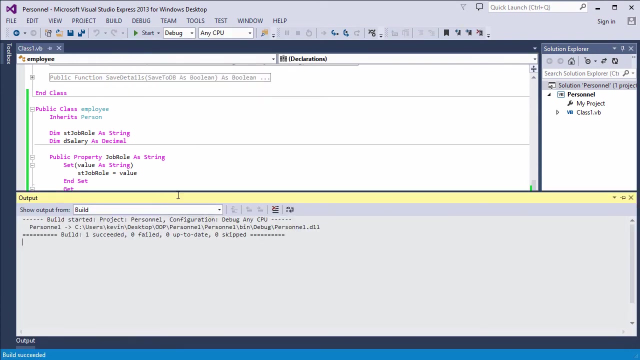 Now I'm going to extend my employee class. I'm going to add some methods and properties which are specific to an employee, Let's say job, role and salary. Let's rebuild the class library And take a look at the front end again. 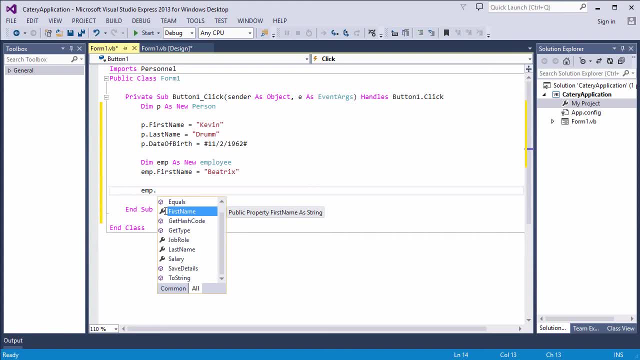 My employee has two extra properties now. Now I should say it's still possible to create a person object directly from the person class and it will have its own original interface. But you can see here that the employee has inherited all of the characteristics of the person. 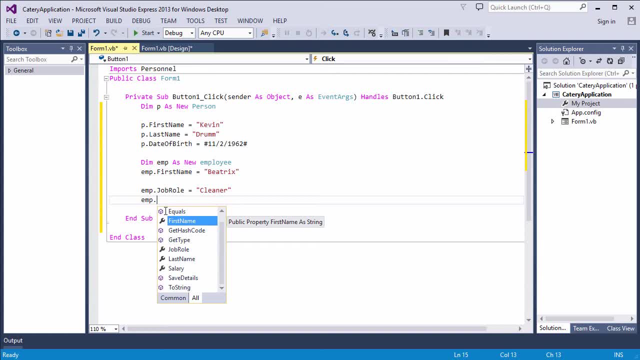 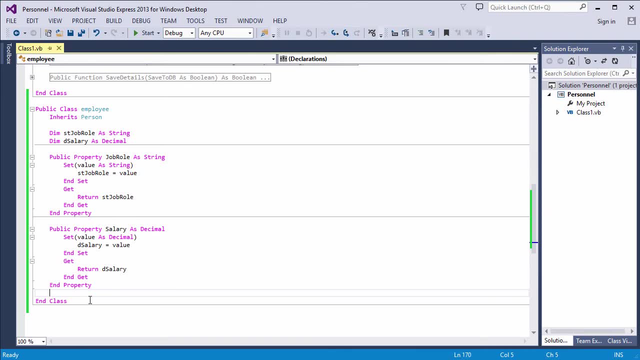 and then it's gone on and extended them with some of its own. Now, suppose I want to code up another class which is a type of employee. I can do that too. Perhaps, for example, I have casual and permanent employees who are different enough to warrant separate classes. 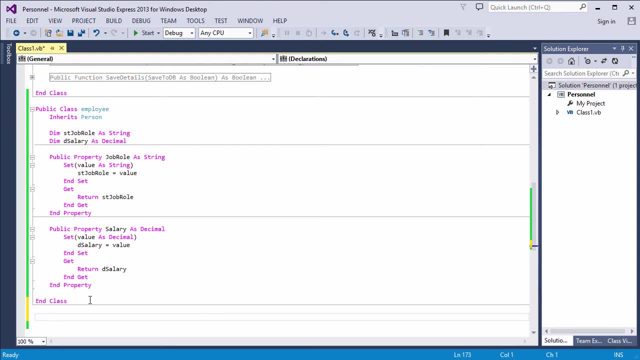 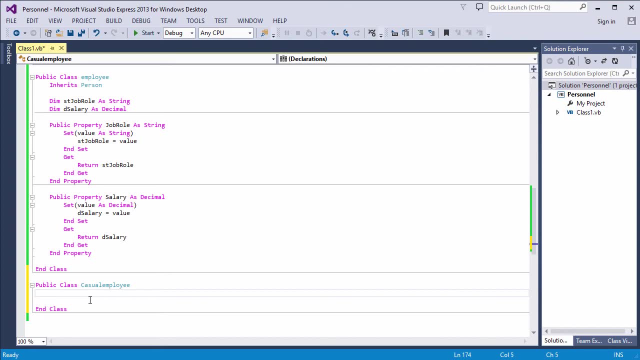 It couldn't be simpler. I write my new casual employee class like this And I can inherit from employee with one command like this. And now I can extend the casual employee class. Perhaps I'll add a property called agency contact. That is the name of the agency that sent this employee to the cattery in the first place. 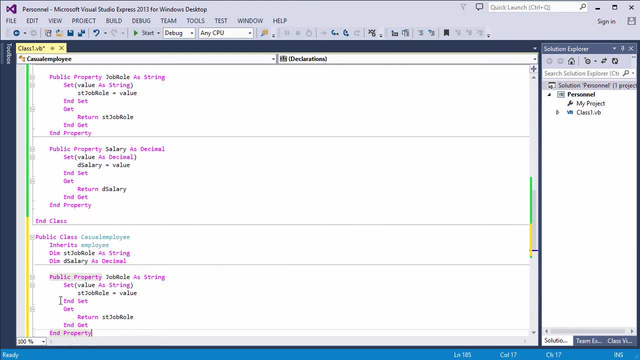 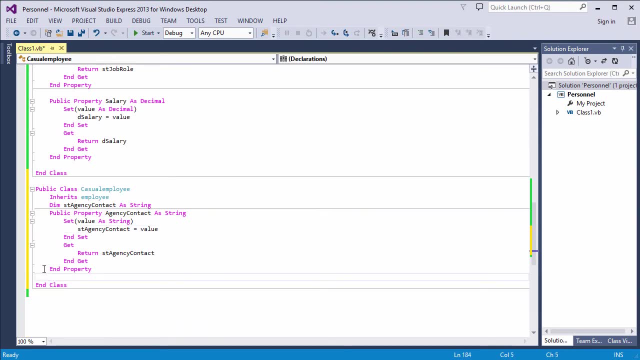 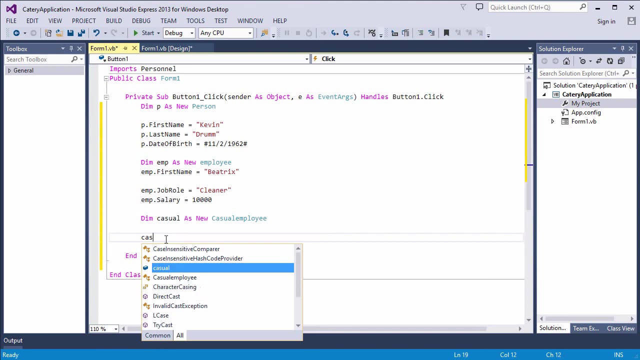 A bit of copying and pasting for speed here And we'll rebuild the library and try this one. And there we have it: A casual employee who has all of the methods and properties of an employee. who has all of the methods and properties of a person. 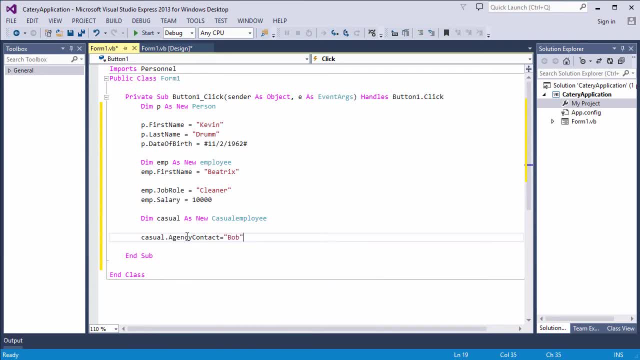 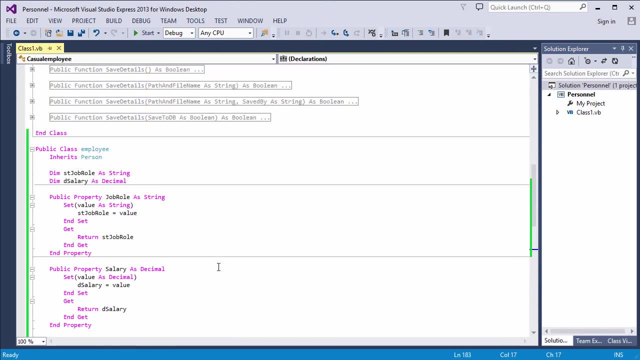 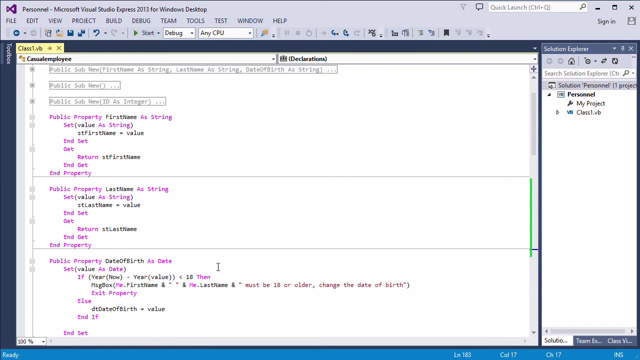 We have a chain of inheritance here. Now let me reiterate this: The real power of inheritance. Suppose I change the code in my person class, Perhaps by adding another property like middle name or nationality, Or maybe I change the way that date of birth is validated. 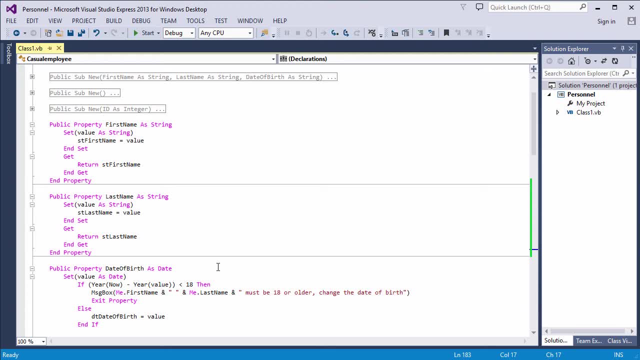 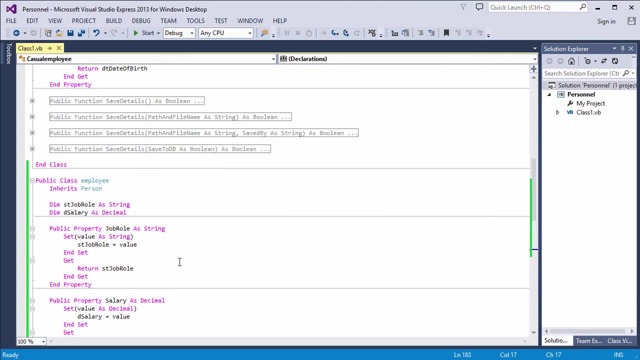 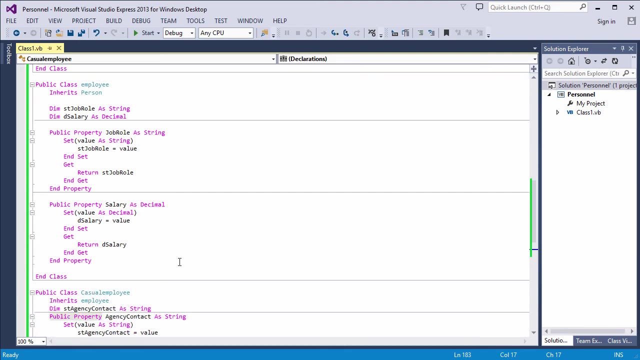 Or the way one of the methods has been implemented. Any changes will be instantly passed on to any classes that inherit from person, In this case employee Indeed. those changes will be passed all the way down the chain of inheritance. This is a good time for some terminology.